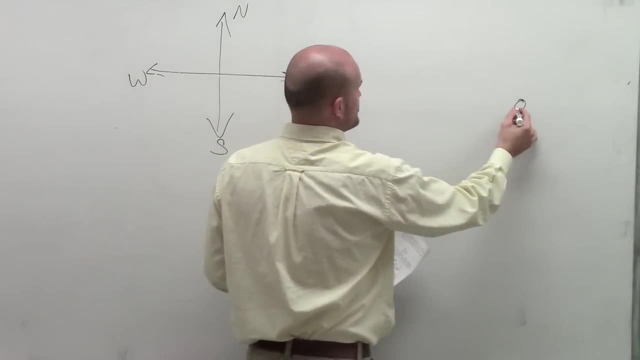 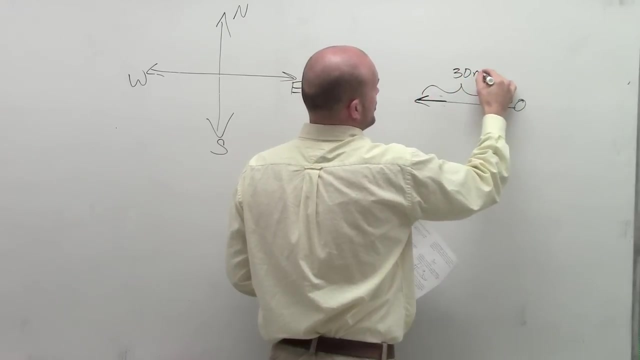 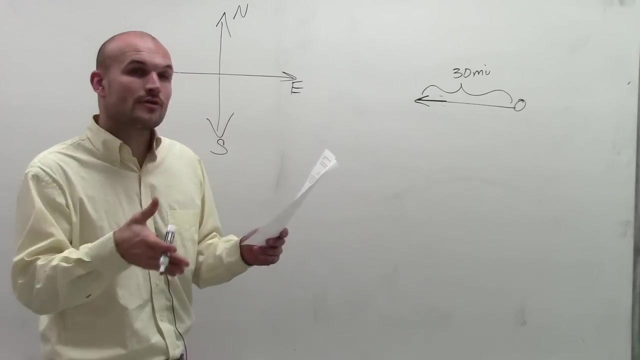 miles. So west is going to be my direction, to left. So I'm going to say due west, and then I'm going to label this distance 30 nautical miles. Then it says the ship changes course and travels south, 30 degree west. 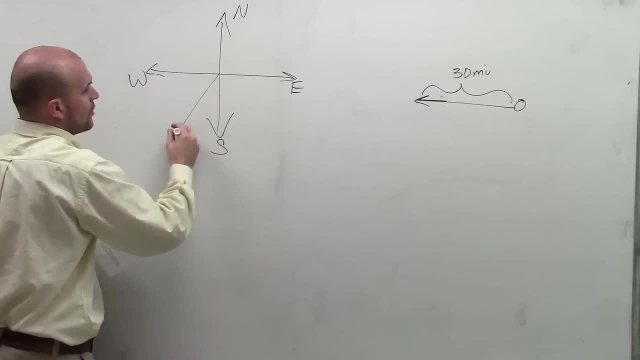 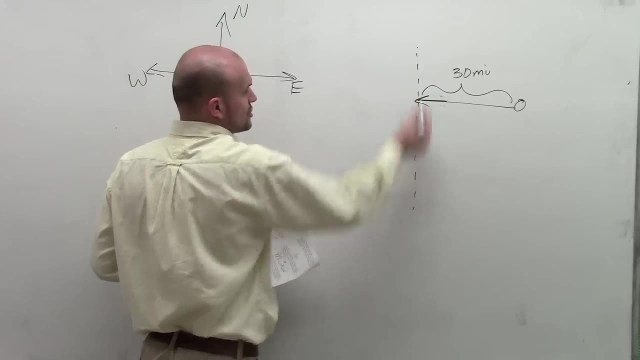 So that means it's going to head in the south direction but then go 30 degrees west. So now it's going to kind of. so if I kind of go back through with my bearings and draw a north-south line, it's going to go 30 degrees in the west direction. 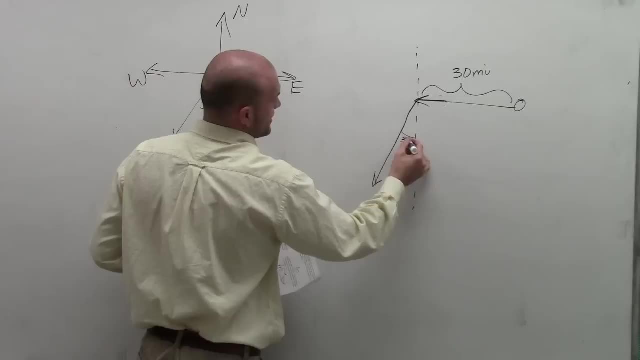 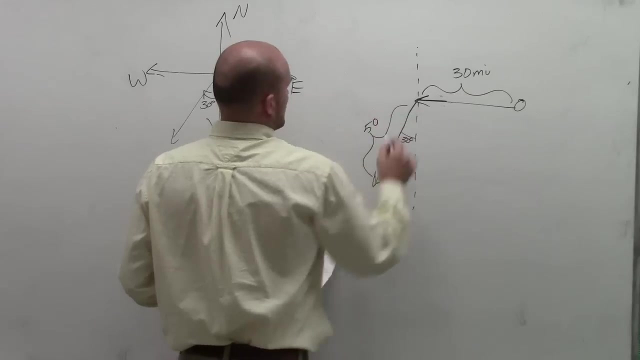 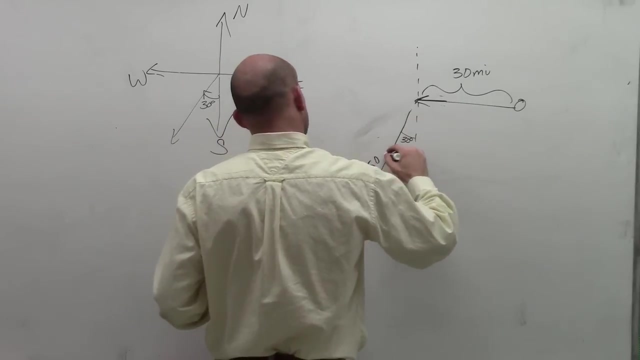 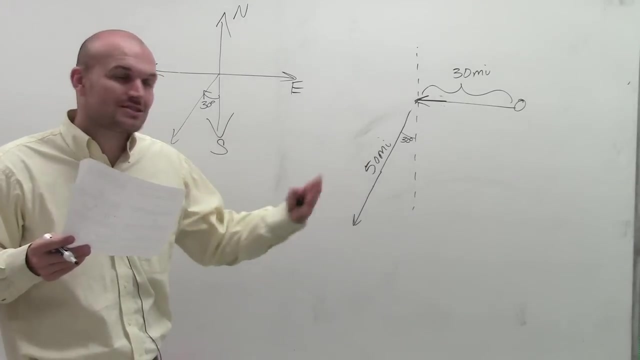 from pointing south. So I could say that angle is now 30 degrees And it's going to travel this distance. That's kind of too big. It's going to travel that distance for 50 nautical miles. Then what they'd like us to do is find the bearing back. 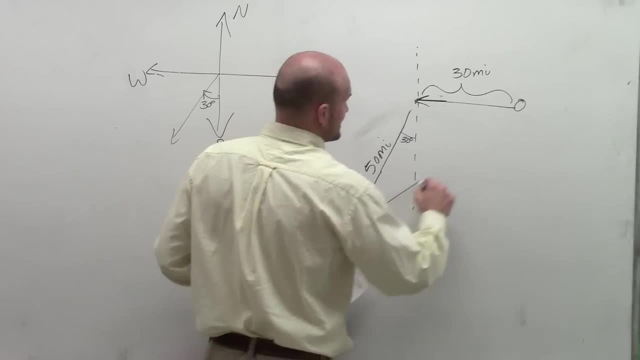 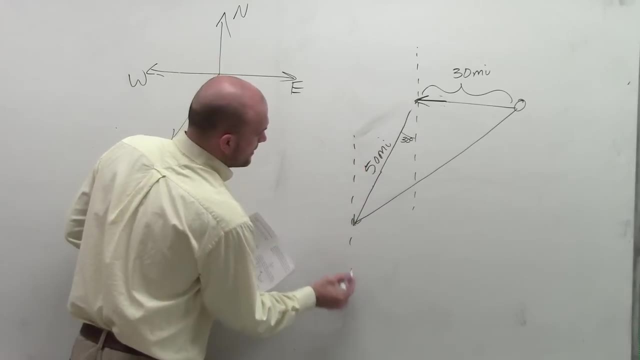 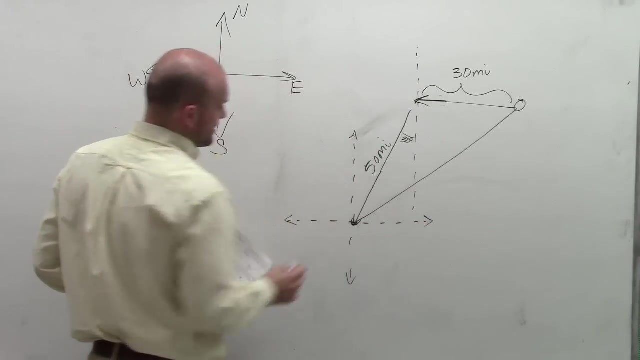 to the port of departure. So they want us to find this bearing that's going to take us back to our port of departure. So what we'll have to do again is we're gonna have to drive a north-south and east-west line from our ending point. 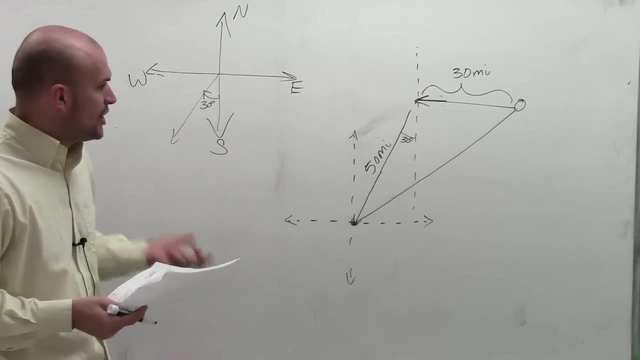 So before we can even do that, though, we need to kind of understand a little bit what are going to be our sidelinks, Or what do we need to figure out? First of all, we need to get a right triangle right. 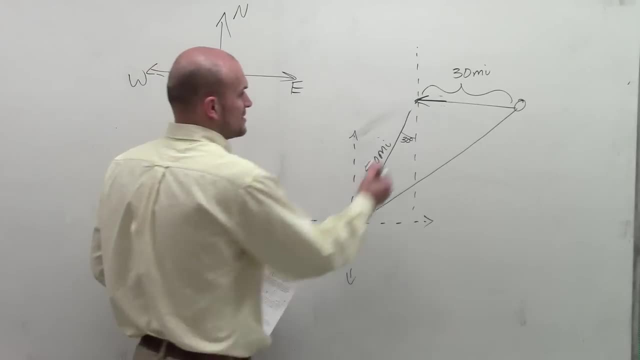 Because, to use our trigonometry, we have to make sure we're dealing with right triangles. So the first right triangle I'm going to do is I'm going to continue this off And I'm going to use this north-south line. 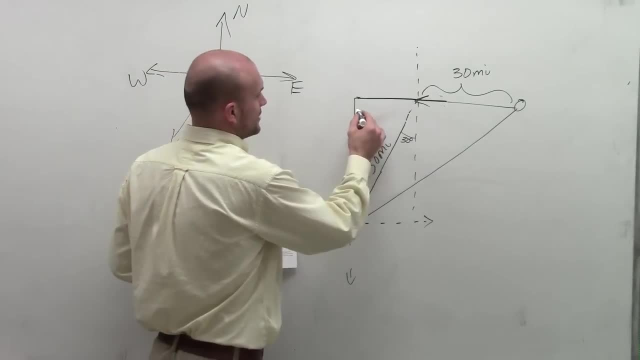 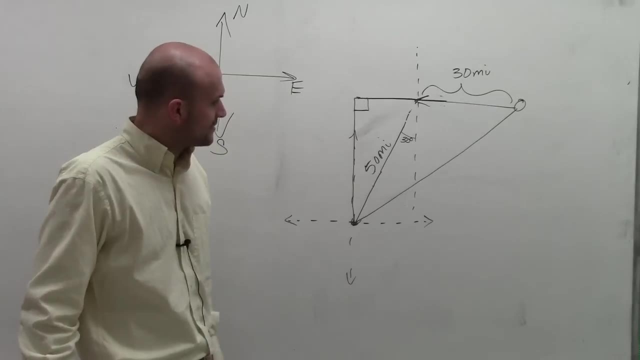 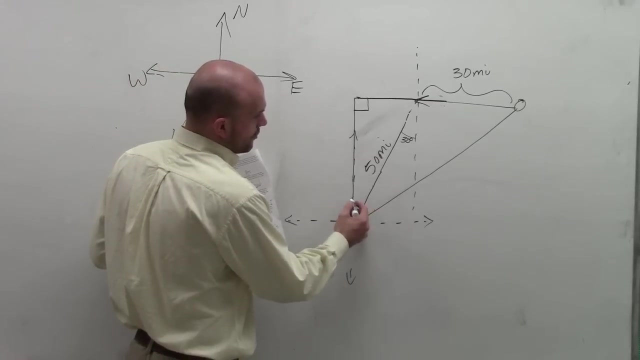 Right south line here and I'm going to create a right triangle here, All right, so I just continued this western and then I contributed my next north-south line. that's going to help me provide my bearing, And what I can do is to find my bearing. I need to be able to figure out, you know what this angle. 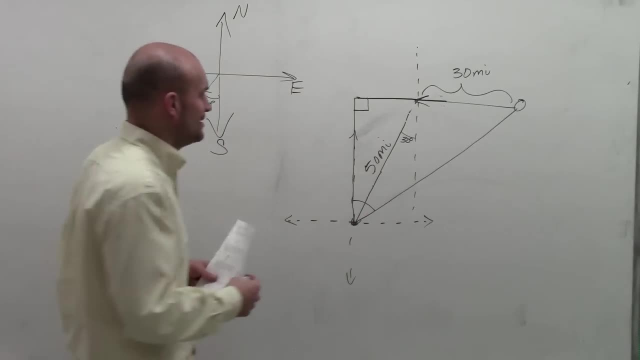 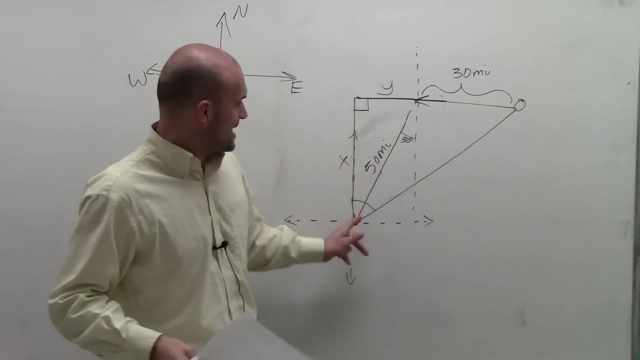 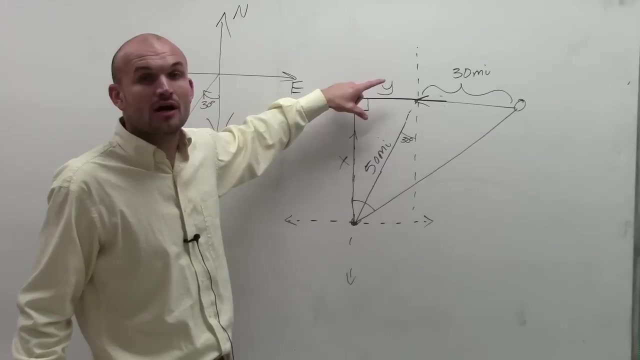 is that I'm dealing with. But before I can figure out that angle, I need to be able to figure out what is going to be this distance and this distance, because right now that's my angle of, that's my angle on my larger triangle, but these two angles are the are side lengths for my 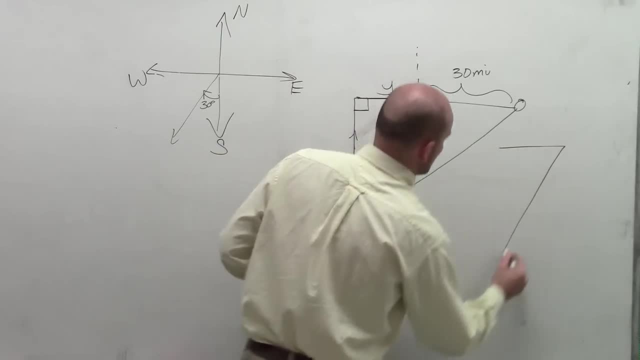 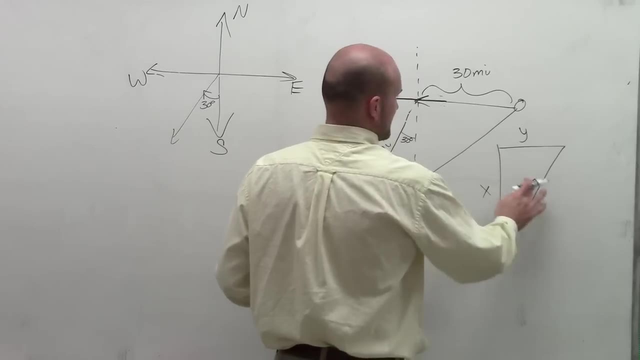 smaller triangle. So what I really have is, you know, if I was to kind of redraw this triangle out here, I don't know what X, I don't know what Y is. The only thing I know is this is 50 miles. 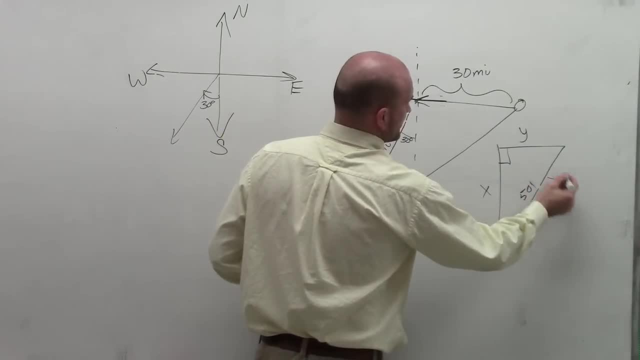 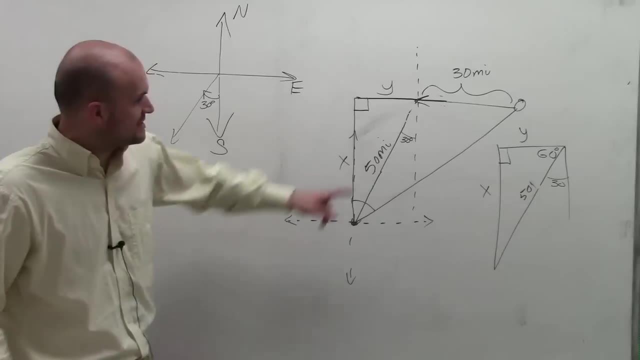 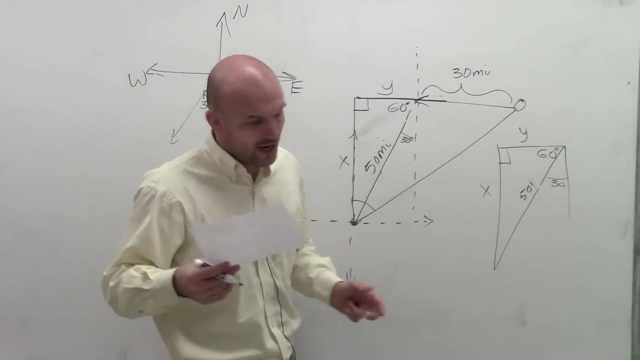 here's a right angle. I know that here is 30 degrees, So therefore this angle has to be 60 degrees. So now what I can do is, since I know that this is now 60 degrees, I can now use my trigonometry to help me figure out what x and y are. 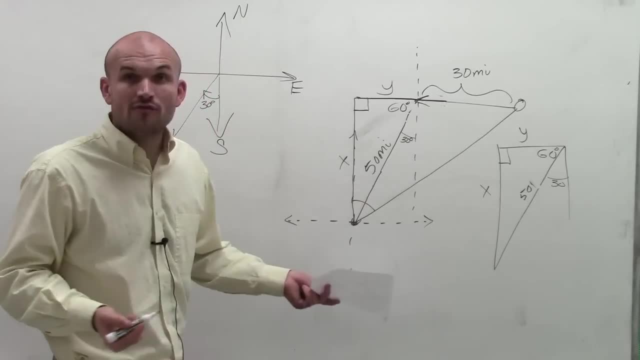 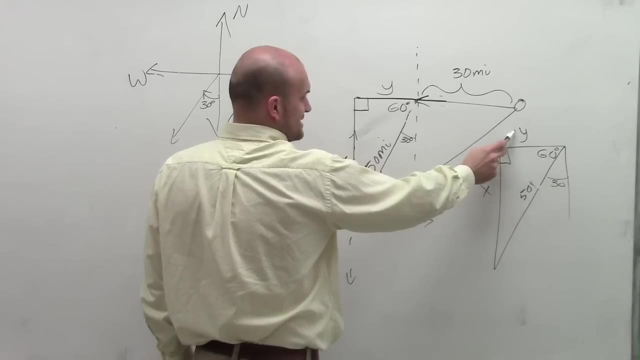 So let's go and write out some statements that we could use to be able to solve for x and y. To be able to solve for, let's do y first. I notice that y is my adjacent side to my angle and 50 is going to be my hypotenuse. 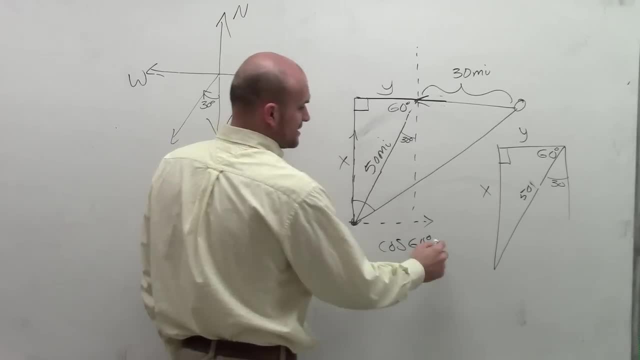 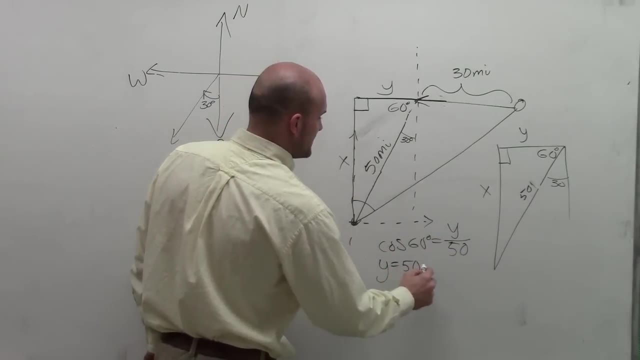 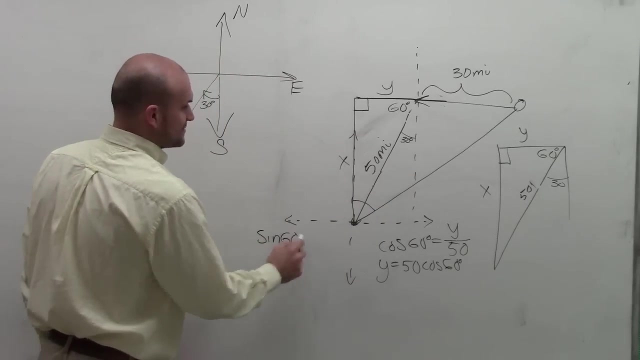 So I could say: the cosine of 60 degrees is equal to my adjacent side over my hypotenuse. So therefore, y equals 50 times cosine of 60 degrees. And then to solve for x I'm now going to use the sine of 60 degrees. 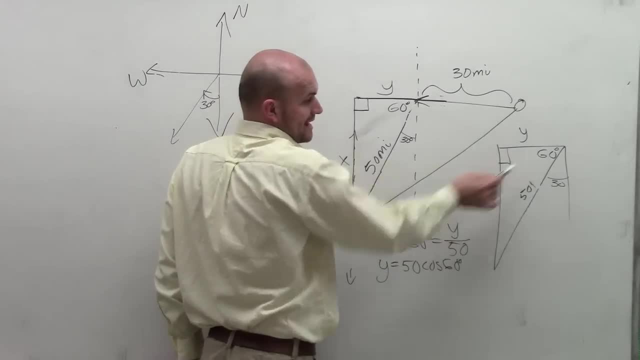 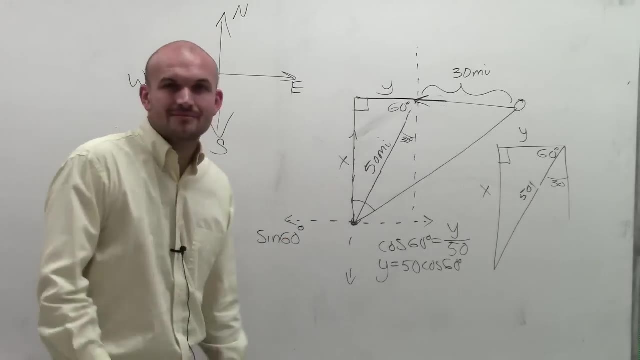 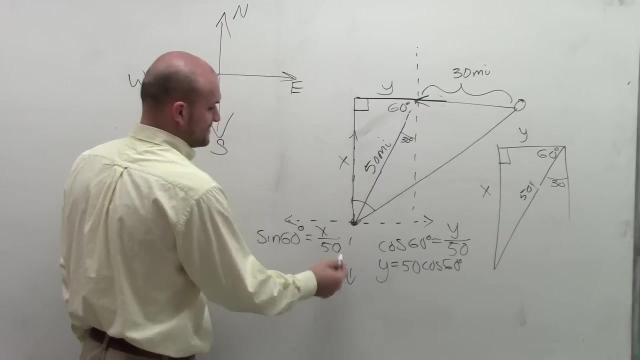 as x is my opposite side from my angle and 50 is my hypotenuse. So I could say: Jacob Newman, can you report to the front office? Jacob Newman, to the front office, please Still make videos. Sign of 60 degrees is equal to x over 50.. 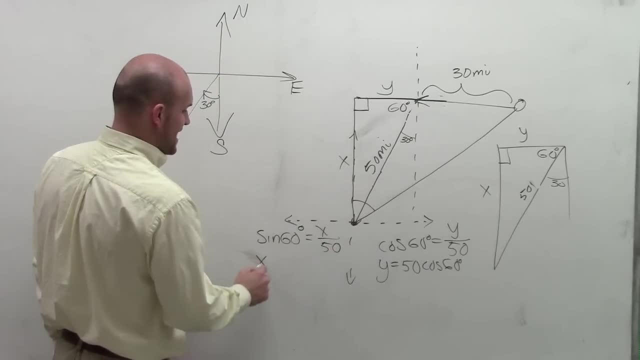 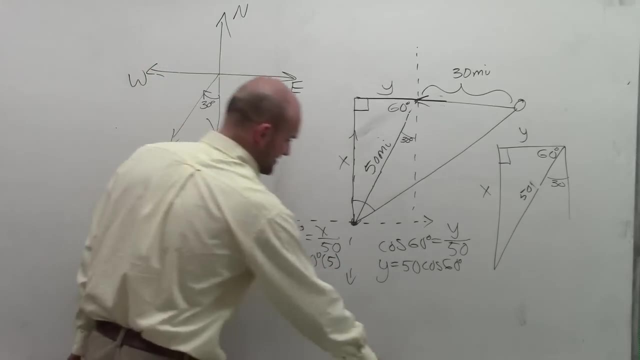 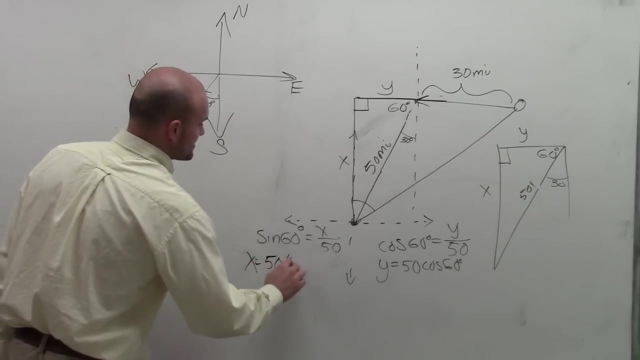 So I multiply 50 on both sides to solve for x, and I could say: x is equal to the sine of 60 degrees times. Let's rewrite that. Let's write it with 50 first. x equals 50 times the sine of 60 degrees. 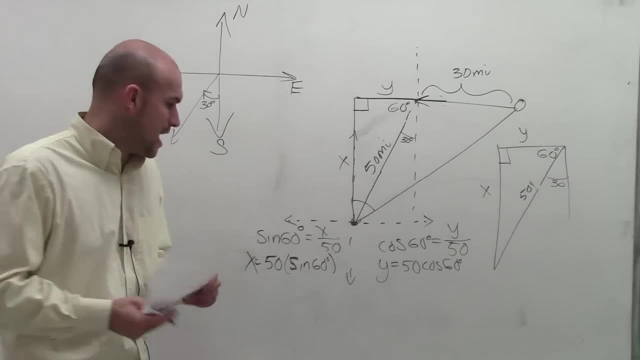 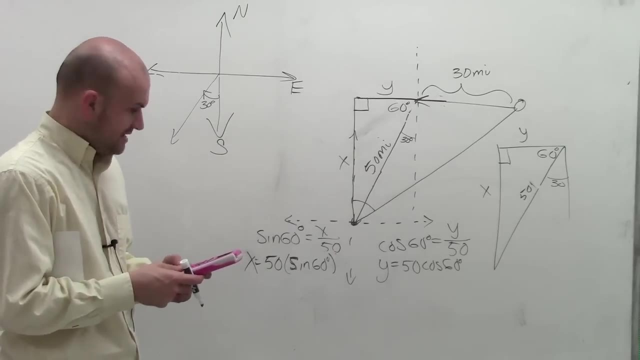 All right. So let's go, Let's go figure these two out, and then we'll go and see how we can, you know, help us figure these out, finish off the rest of them. So what I'll do is I'll do 50 times the sine of 60 degrees. 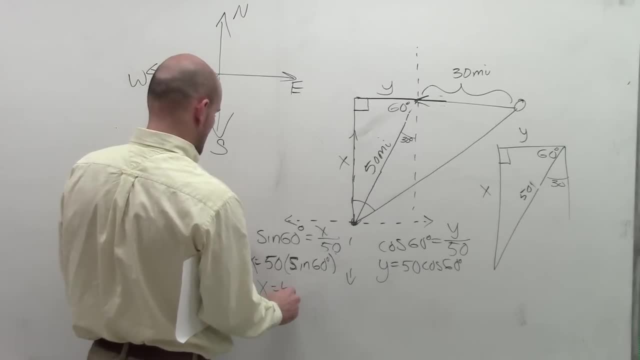 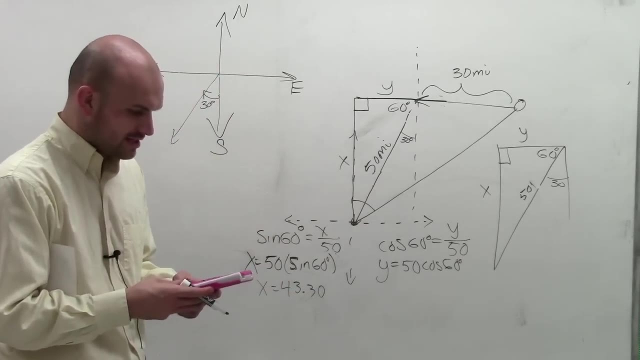 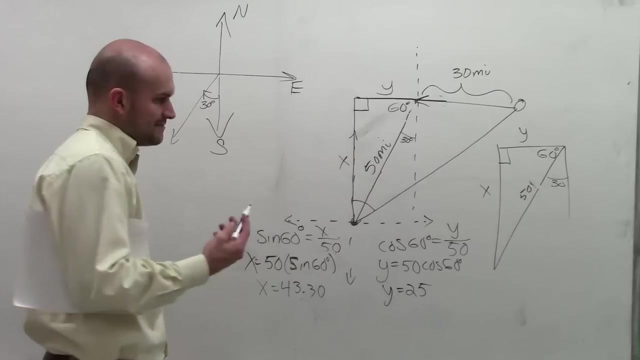 and that's going to give me x equals 43.30.. And then I'll do 50 times cosine of 60, and that's going to give me 25.. All right, Oh, obviously, cosine of 60 would be 1 half.